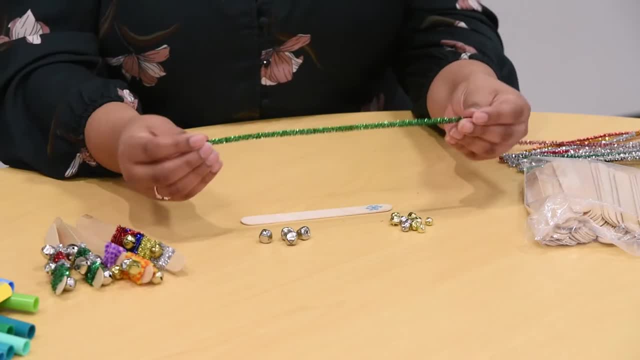 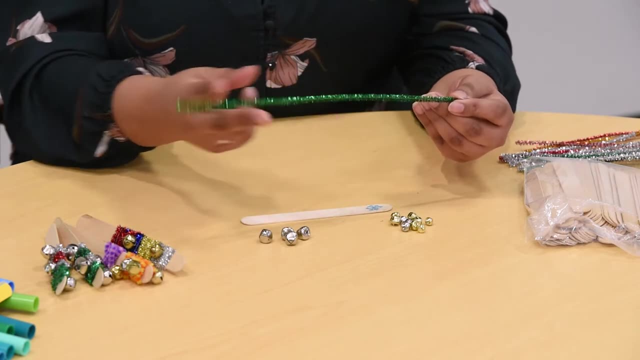 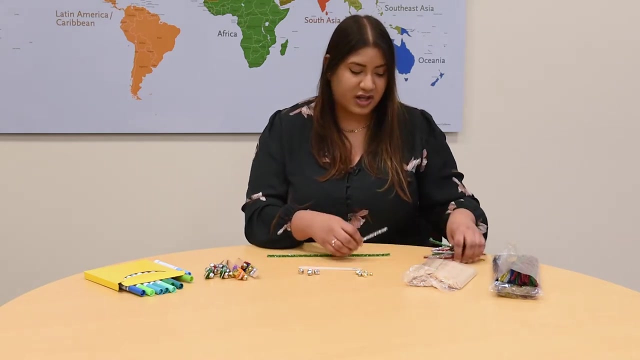 to grab my popsicle stick. here You can grab any color of pipe cleaner that you want. You just want to grab a scissor and just cut it right down the middle and then you have some fun. easy to grab pipe cleaners here. Now I'm going, and you can pick some colors to make it a little bit more. 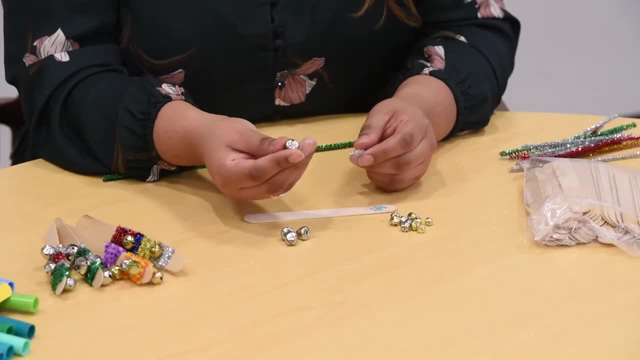 festive. so I'm going to grab one of my larger bells here And you're just going to simply turn it around. you're going to pull it all the way around and you're going to pull it all the way up And on your feet, you're going to grab this hair pin and you're going to pull it up. 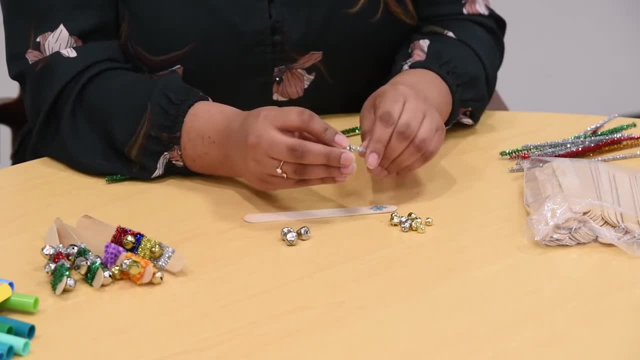 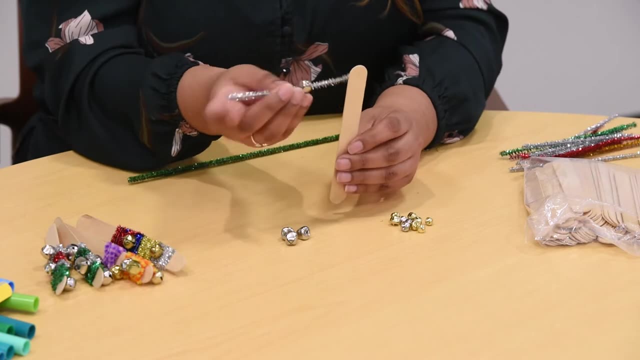 and you're going to pull it up. and you're going to pull it up real good into the spiral And you're going to see a hoop there and you're going to place it right down the middle and easily slide that in. Then you're going to grab your popsicle stick and you're just going to put your bell right. 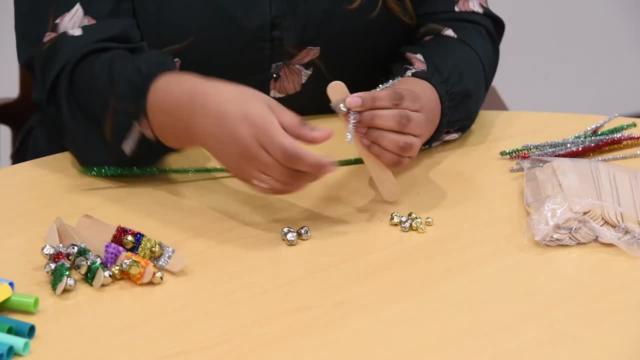 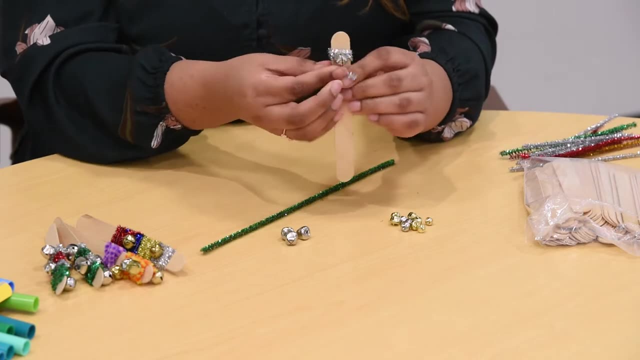 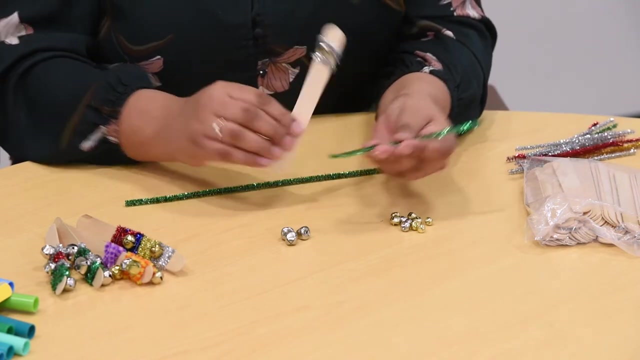 down the middle and you're going to wrap upwards. there we go, and you're also going to go downwards- Very easy, And there you go. we've got our first bell on. Now I'm going to pick a different color. I'm going to go with green. 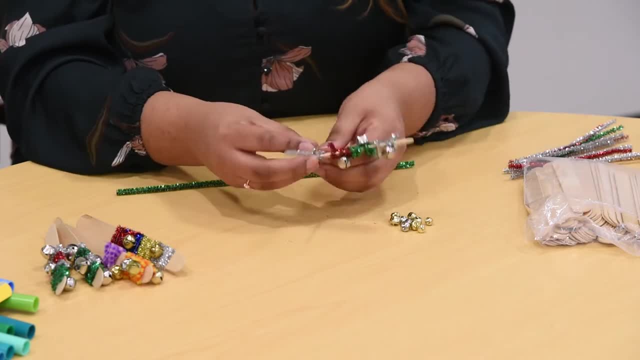 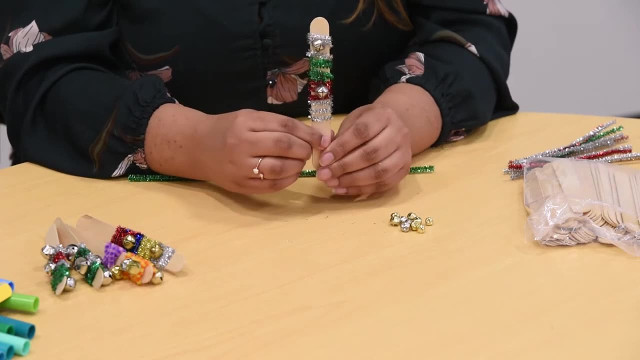 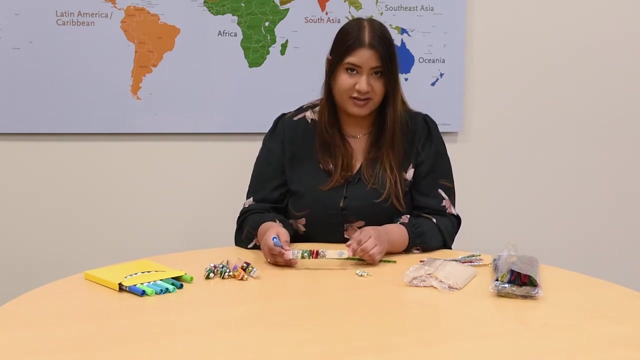 So there we go now. we've got our sleigh bells, you've got two bells on one side and two bells on the other, And you can grab a marker, and what I've done here is a fun little snowflake, but really you can draw anything you like. 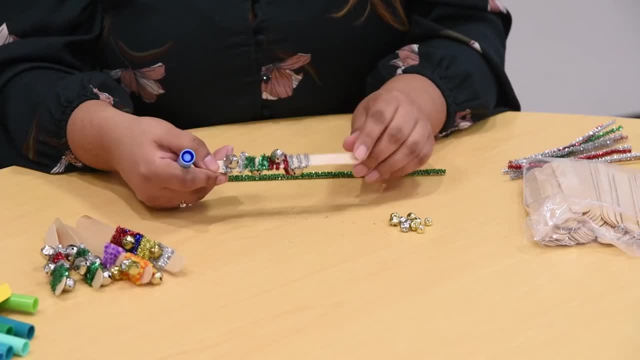 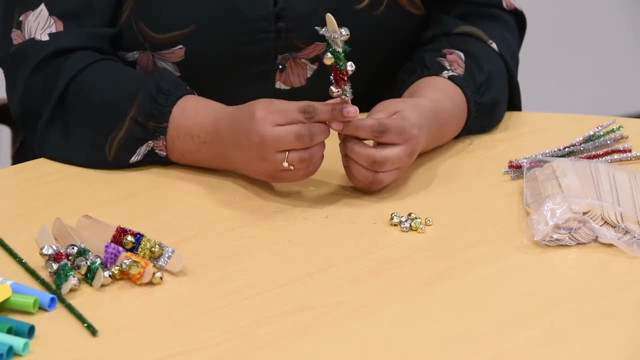 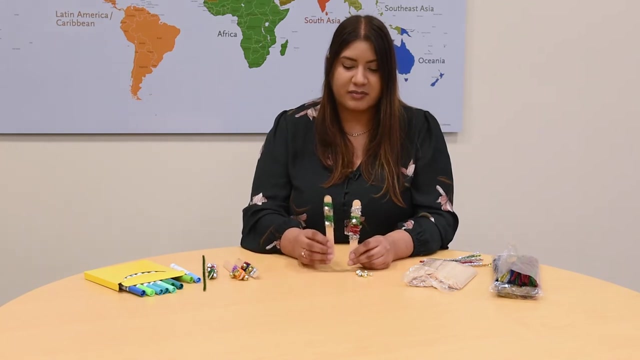 So just be creative and mark up your popsicle, stick with the extra space here, and then you've got a really fun popsicle or sleigh bell. So, as you can see, these bells are about medium size, But I've got some bells that are even bigger and can make a different sound there. 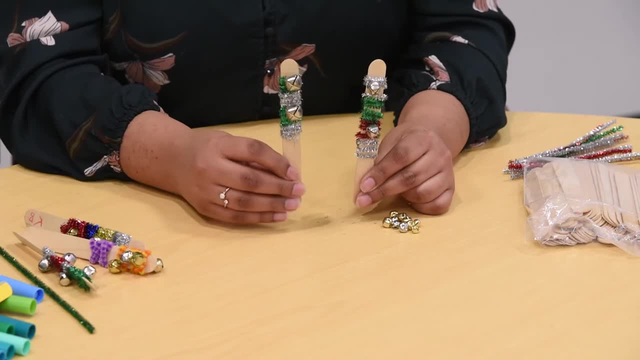 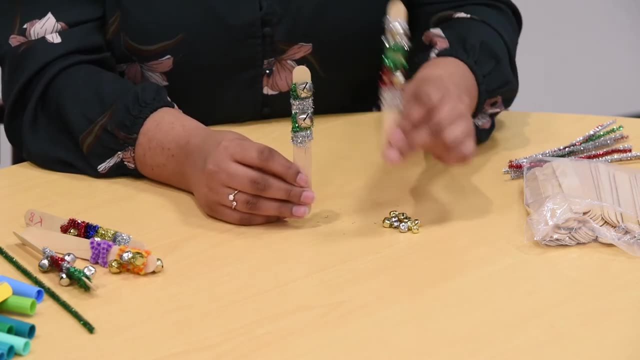 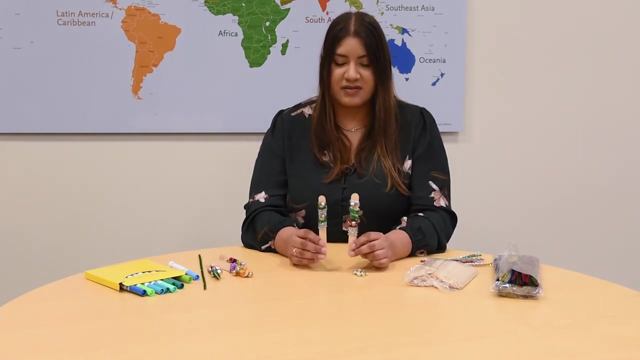 So let's see what they sound like. So I'm going to play this one first And then we're going to play the other one. Can you hear the difference there? They just create a little bit of different sounds. but then when you play them together, 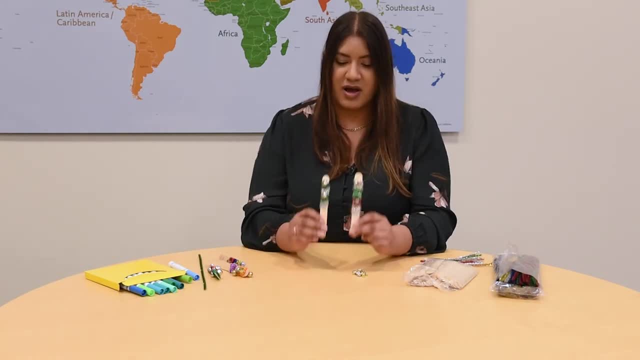 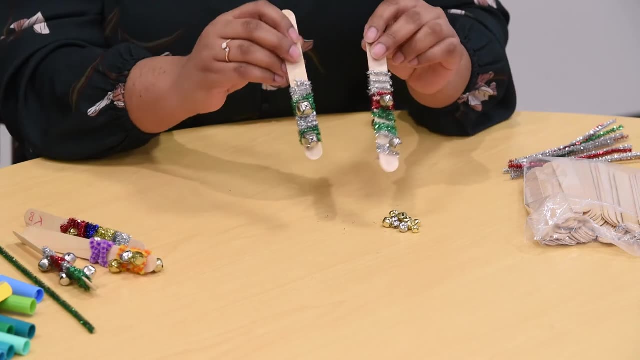 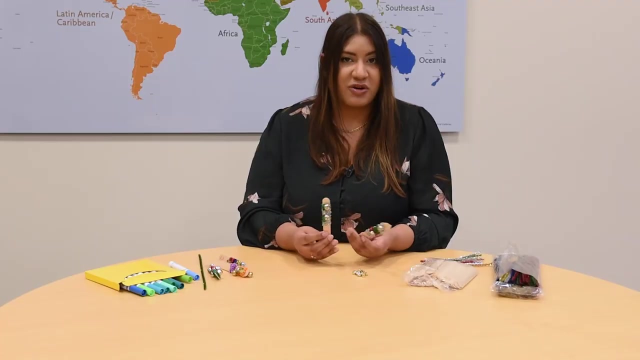 you can get a really fun combination. So you can either go Go up and down, Or you can flip them upside down as well, and you can do the same thing. And then what you can do is, at home, just pick your favorite song- maybe a holiday song- and 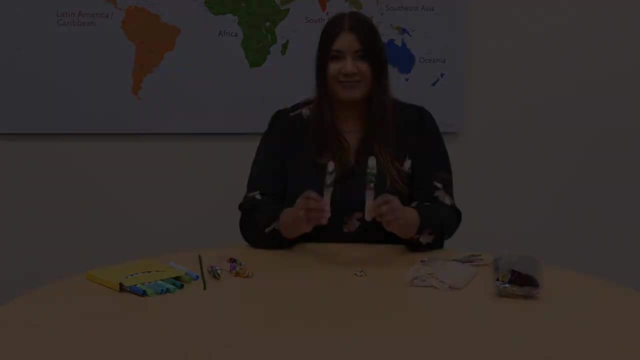 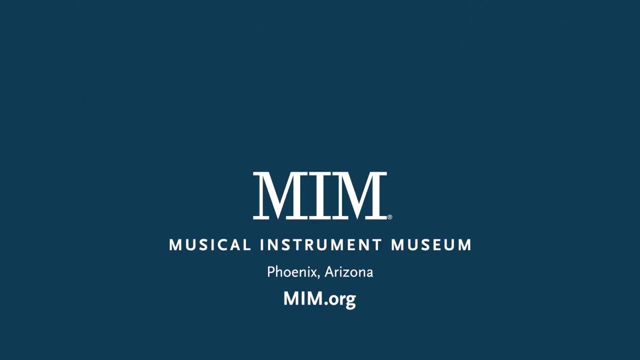 just jam along with your sleigh bells And that's pretty cool.